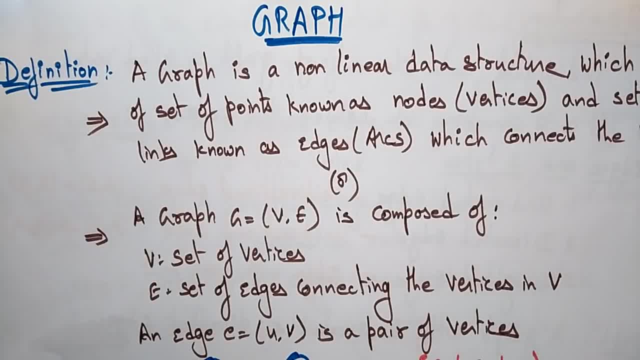 Hi students, welcome back. Coming to the next topic in the subject, data structures- was graph. So far we have discussed about the trees. Now let us see what is a graph. A graph is a non-linear data structure. The one thing you have to remember that this graph you 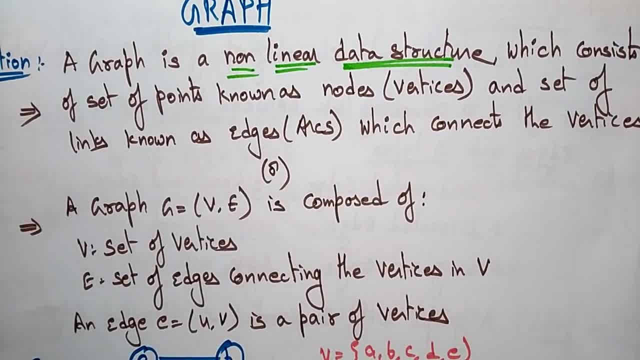 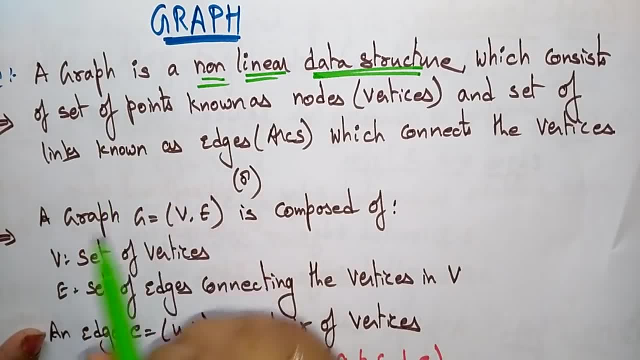 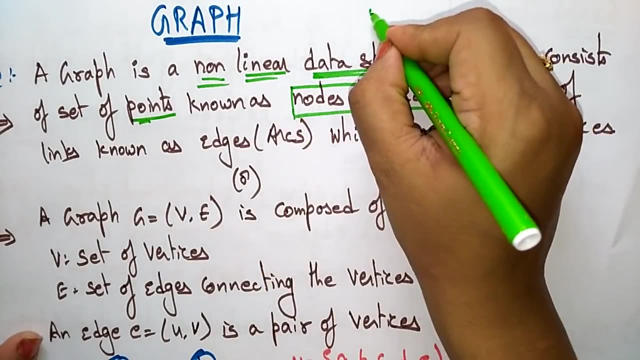 call it as a non-linear data structures, whereas stack queues, those are the linear data structures. So graph is a non-linear data structure which consists of set of points. A set of points we call it as nodes, or vertices, Means it consisting of some set of points, that is, vertices and set. 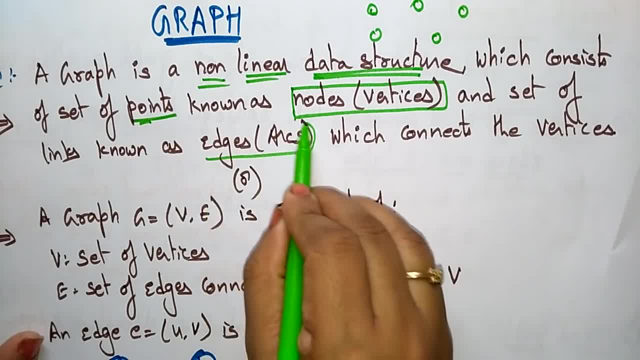 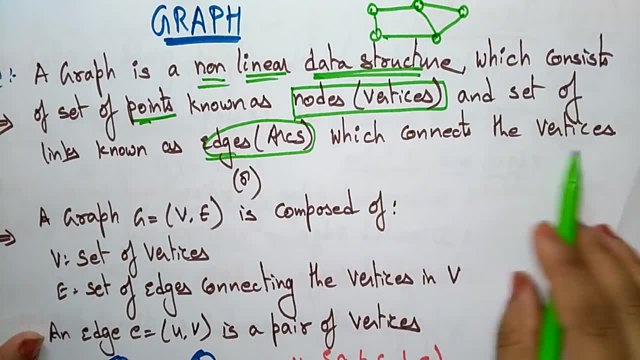 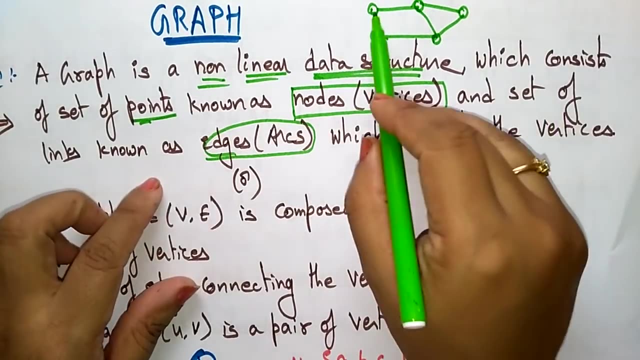 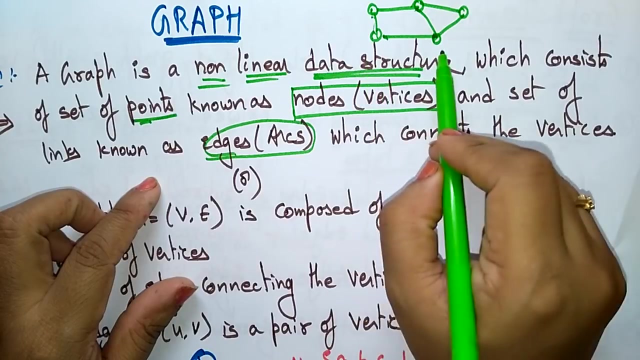 of links, known as edges. Edges or arcs means link, means connecting between the nodes, which connects the vertices. A definition of a graph: A graph is a non-linear data structure which consists of set of nodes and the set of links which you call it as an edges, which connects the vertices. Or you can tell: 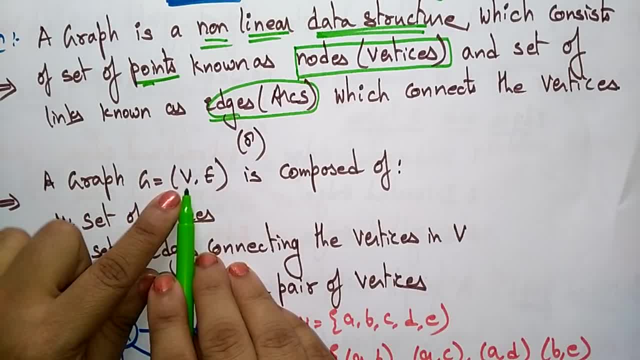 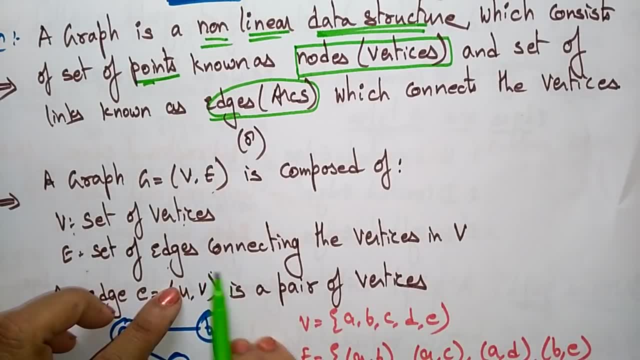 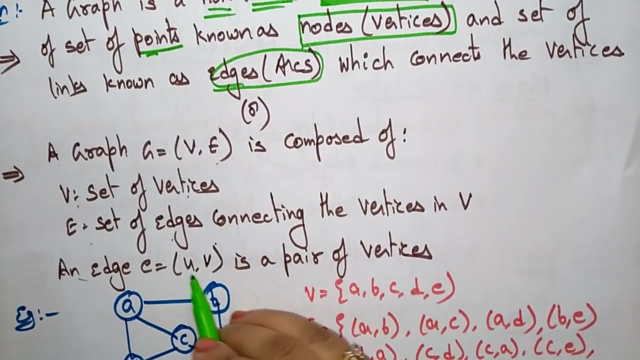 a graph G is a set of vertices and edges, is composed of where V is a set of vertices and E is a set of edges connecting the vertices in V. And here we have a graph G, which is a set of vertices and edges. Here an edge, E is nothing but is a pair of vertices, That is, this is suppose let us take. 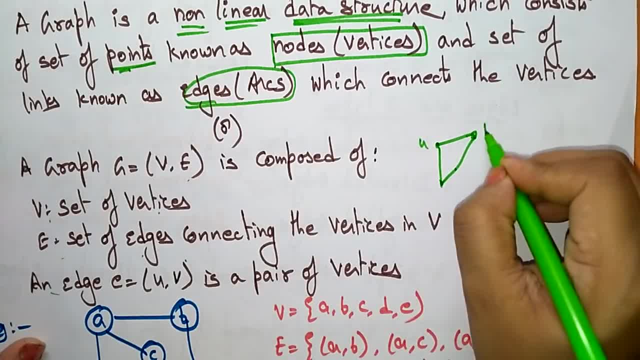 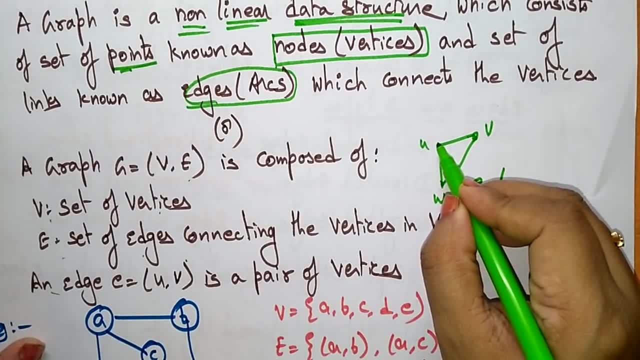 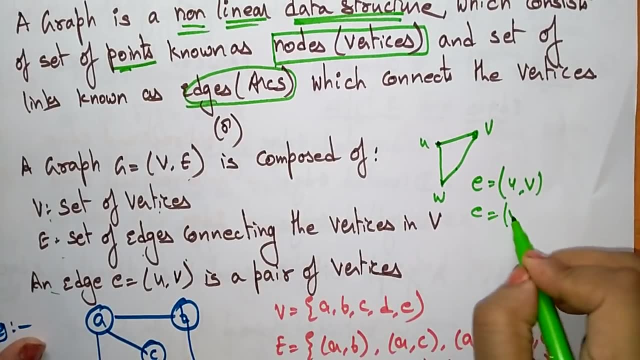 this is an edge. U, V, W, These are the vertices. So the edge E is nothing but this pair of vertices, U and V. This acts as one edge, Or E is equal to V, W. So this is one edge and this is one edge. 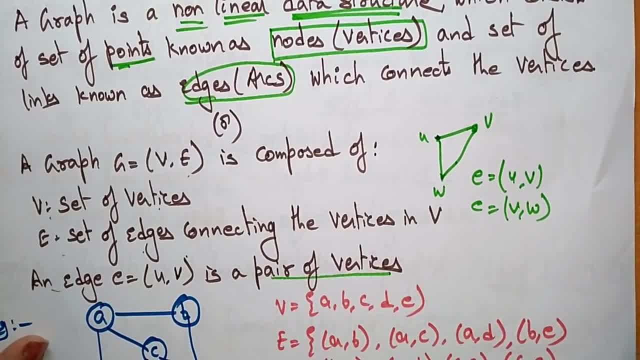 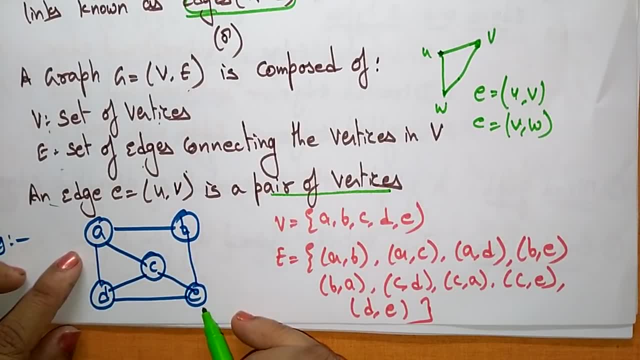 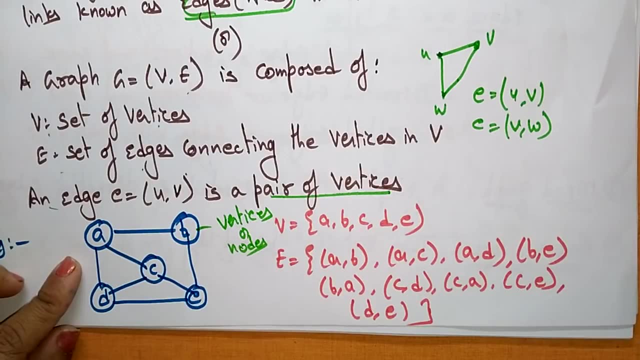 So edge is a pair of vertices, So let me show you a simple graph. So here, what are the A, B, C, D, E, These? you call it as vertices, or you also call as nodes. And coming to these links, These links, you. 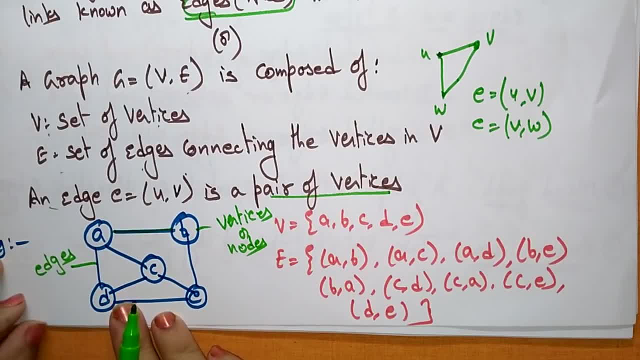 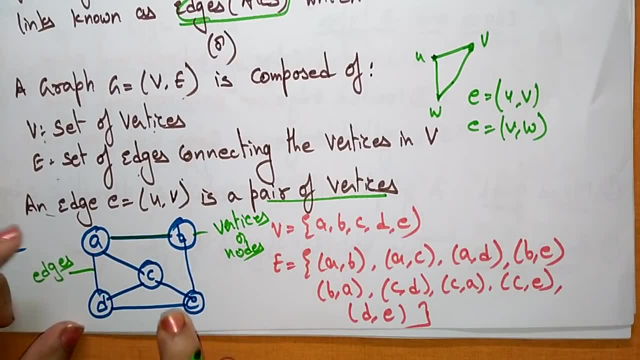 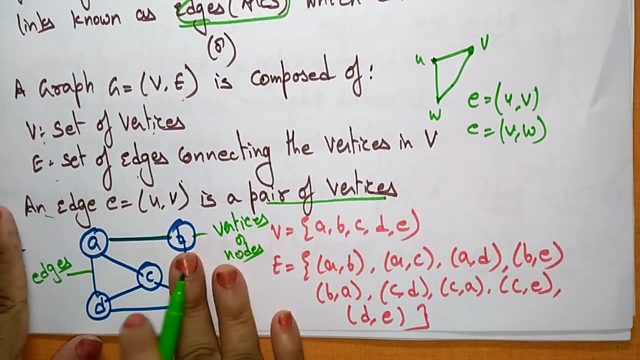 call it as edges or you call it as arcs. So here the set of vertices are A, B, C, D, E. So this graph consists of five vertices. And what about the edges? So this is a. it is a non-directed. 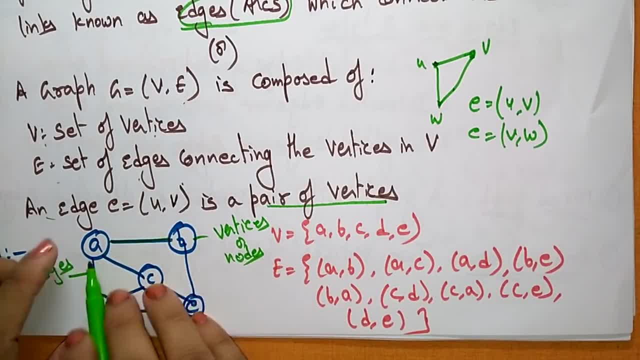 graph means undirected graph. There is no direction, So it's a two-way direction: A to B or B to A. Both are the same. So A, B, A, C, A, D, Next B, B, A, B, E, Next coming to C, C, A, C, D, C, E, D E. So these are all these. 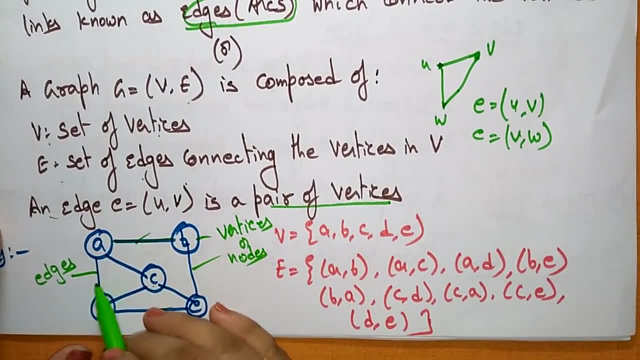 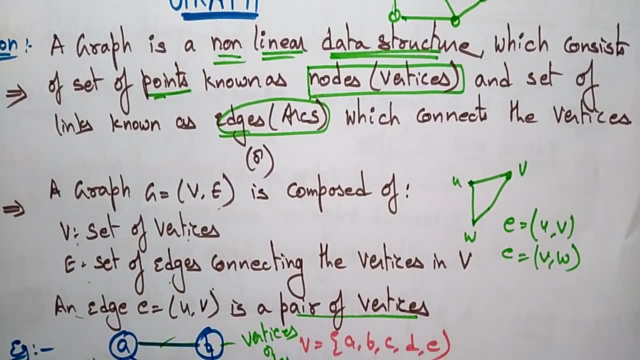 So this is a set of edges. You call it as edges. These are all the edges. So that is the definition of a graph. Whenever you ask about what is a graph, you first tell graph is a non-linear data structure and try to write this definition with an example. 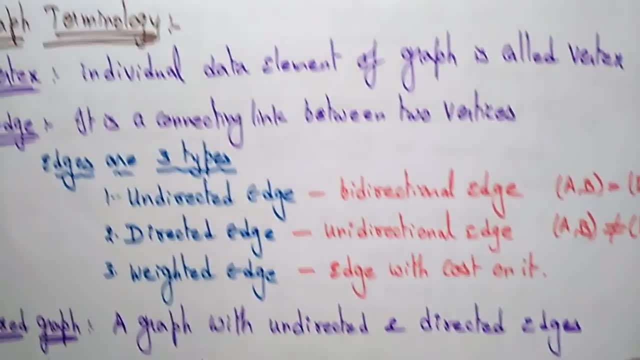 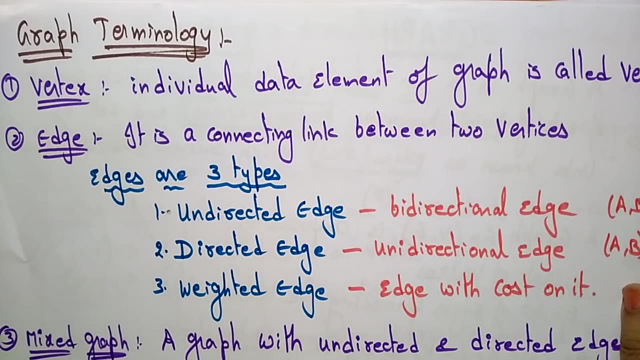 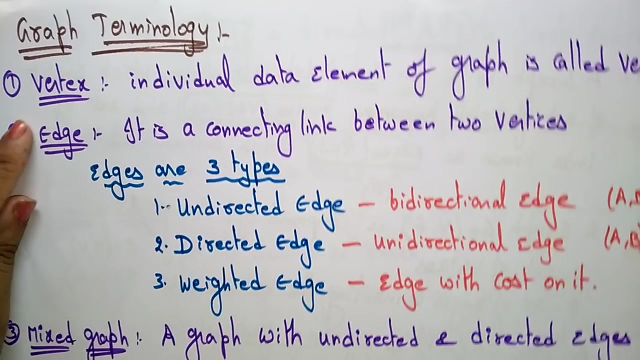 Next, coming to this, some terminologies that you use in the graph. Let's see the graph terminologies. So, while you are discussing about the graph, you came across some words. Okay, some terminologies. Now let's see vertex. i already said a vertex is nothing, but it is a node. individual data element of a graph is called. 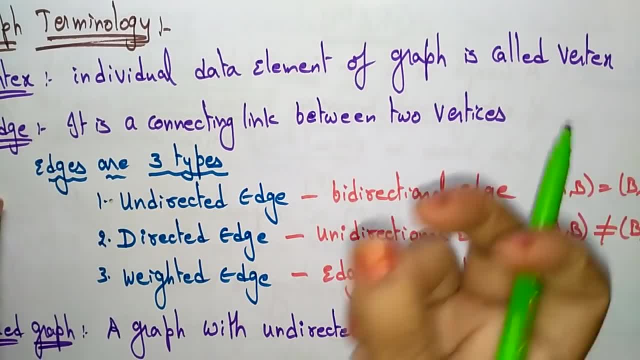 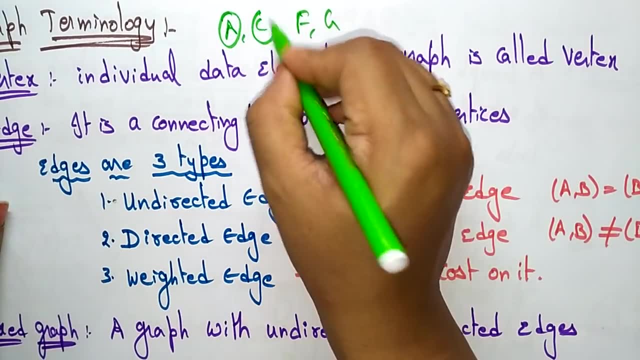 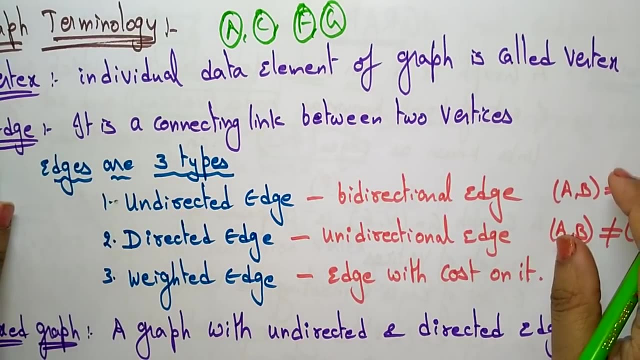 vertex. so whatever the data that is you are providing, so that the individual data element, suppose a, c, f, g, these are the data elements, in that each element you call it as a vertex. so individual data element of a graph is called vertex. you also call it as a node. 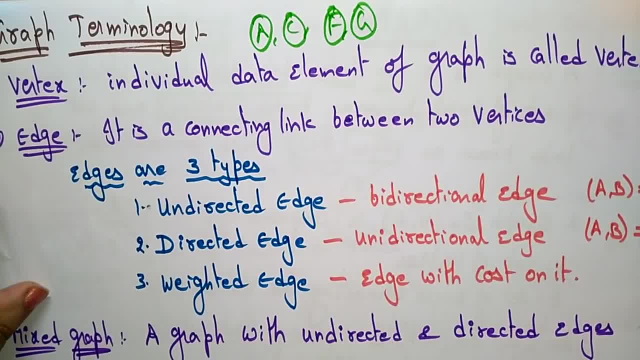 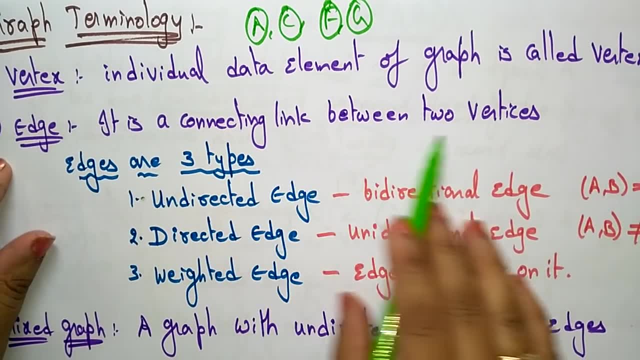 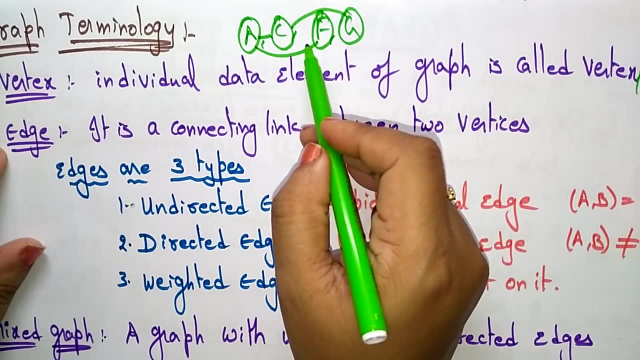 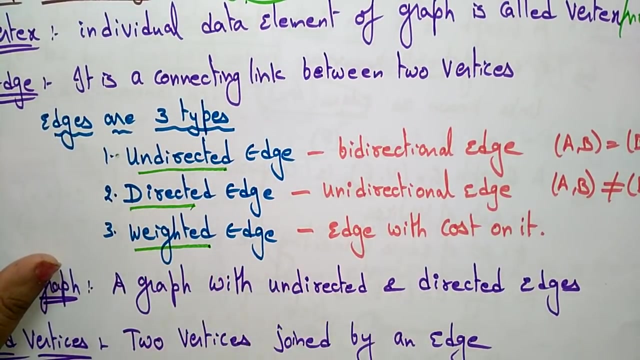 next coming to edge. the next terminology is edge. edge is a connecting link between two vertices. so it's just a connecting link between two vertices. it's just a link. so this edges is of three types: undirected edge, directed edge, weighted edge. so what is this? undirected edge, directed? 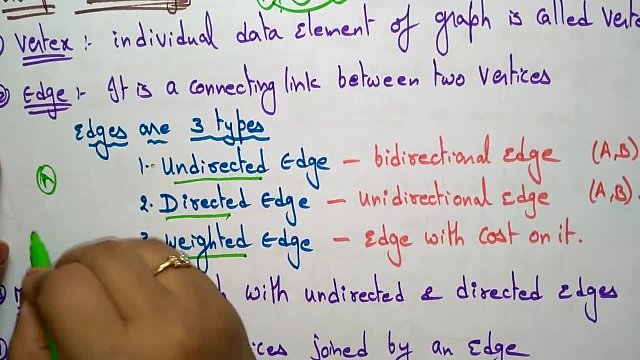 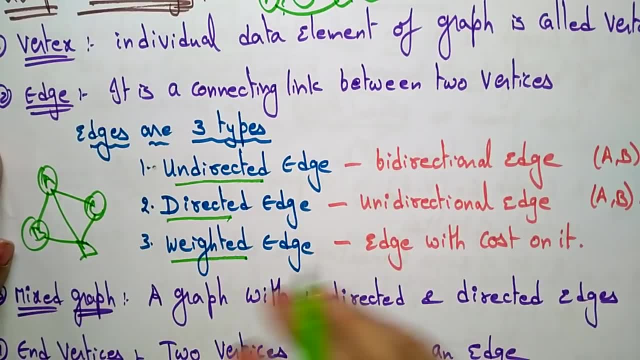 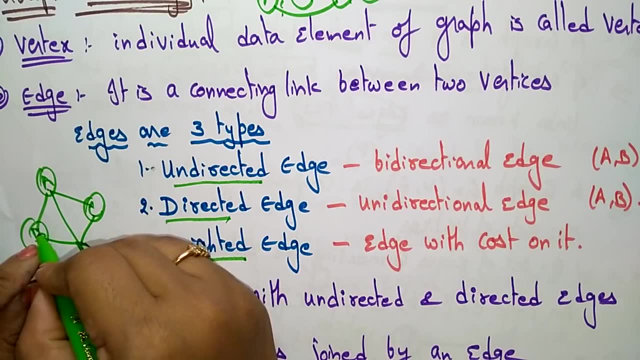 weighted edge. so let me take, suppose, a, a, a, a, a, b c d. so this is a graph b c d. so this is a graph okay. so this i call it as undirected graph. okay, so this i call it as undirected graph edge because there is no direction from one vertex to another vertex. 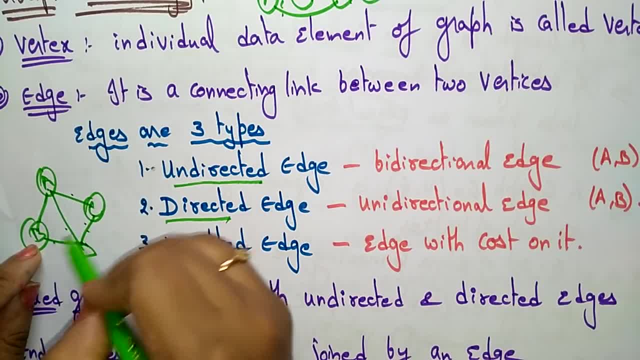 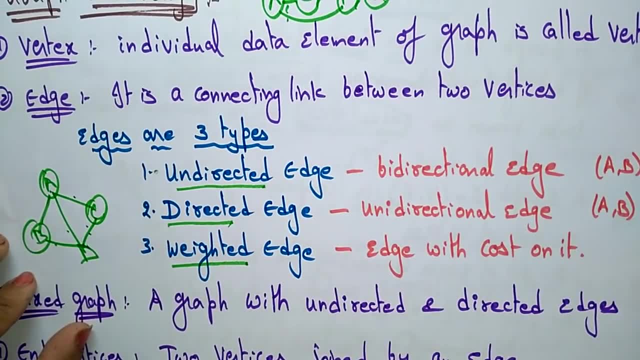 means here the edge. whatever the edge is present here, this edge doesn't have any direction, that is, it is a bi-direction. if no direction is there, you can take it as a bi-direction: a to c or c to a, b to a or a to b. 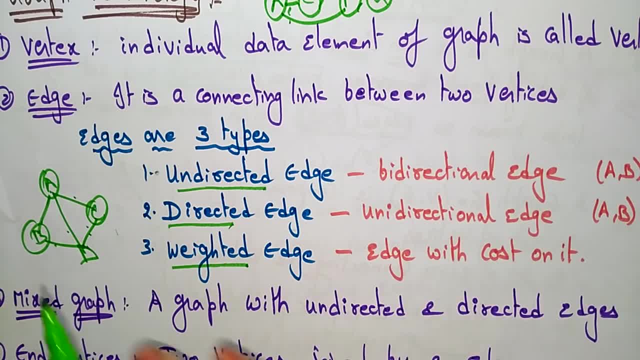 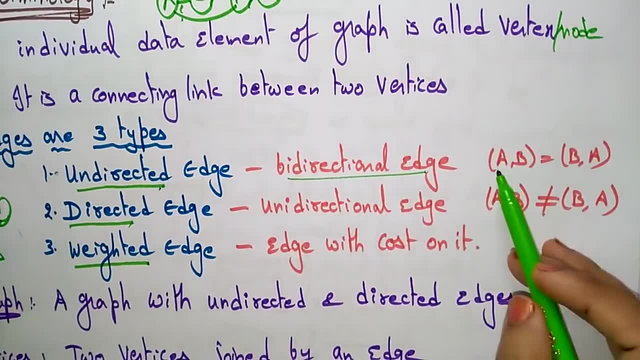 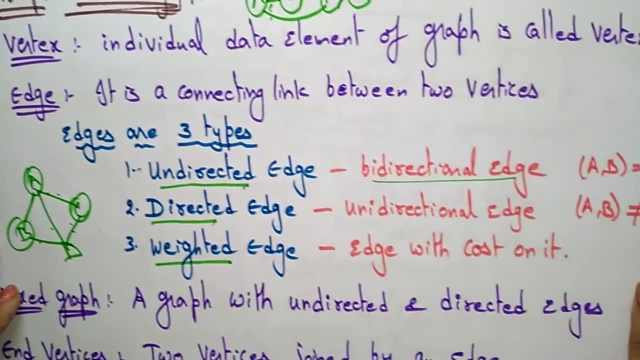 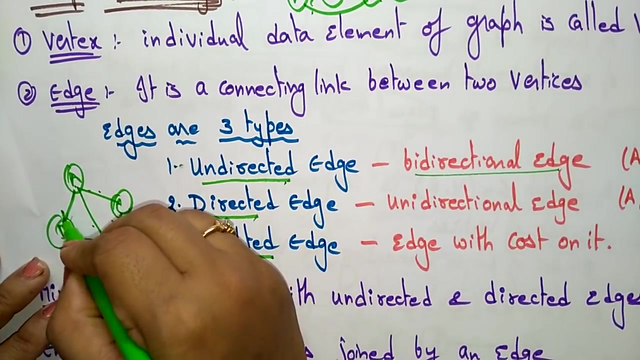 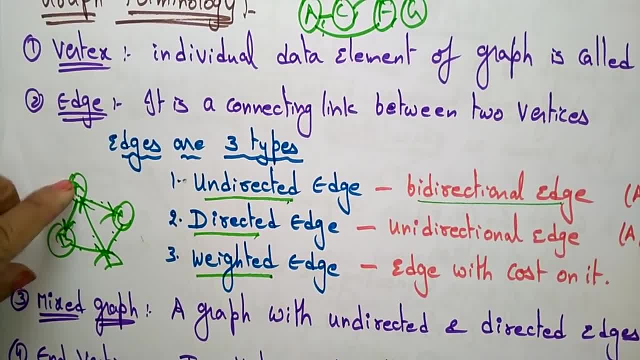 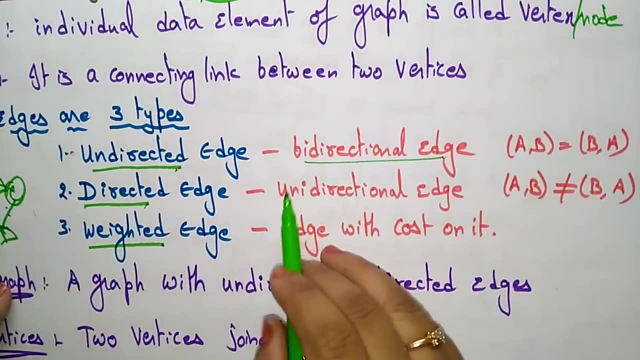 as a direction. so you can go from a to b, but b to a is not possible because there is no direction from b to a. you can go for a to b from a you can reach b from, but from b you can't reach a because there is only one-way direction. so the unidirectional edge. we call it as a unidirectional edge, so here ab is. 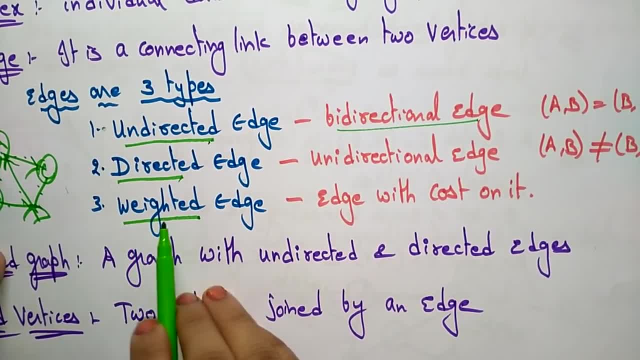 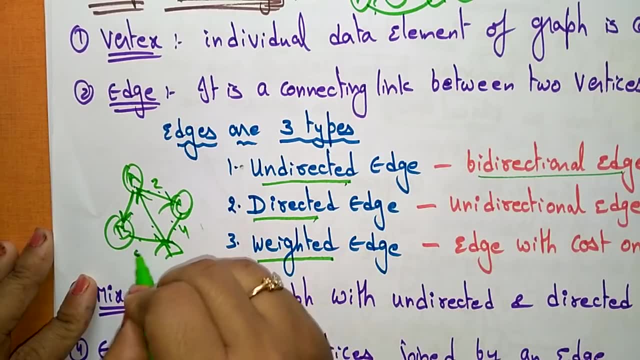 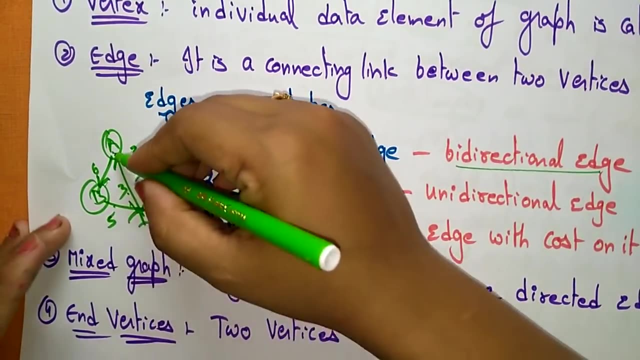 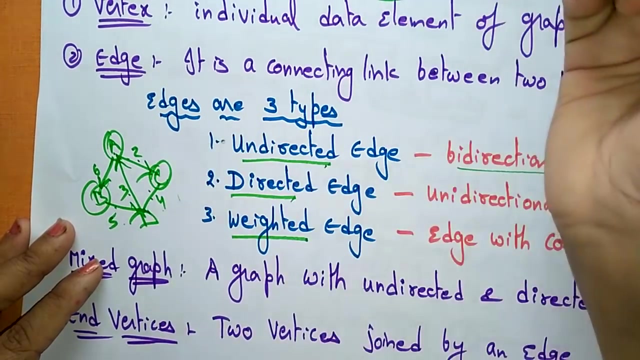 not equal to ba. the next type of edge is a weighted edge. weighted edge means edge with cost on it. let me take 2, 4, 5, 6, 3, like that means that edge will hold some weight. if you want to go from a to b, the weight of this edge is 6, and b to d, the weight of the edge is 5. okay, now coming to. 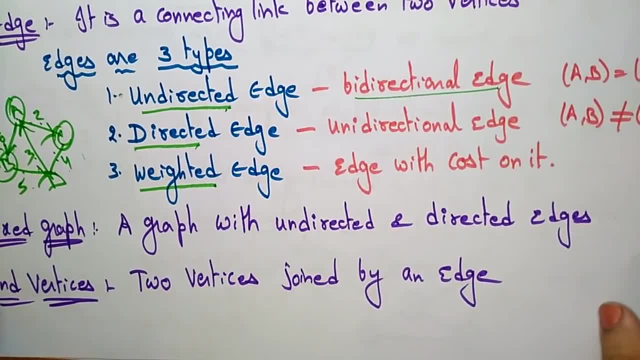 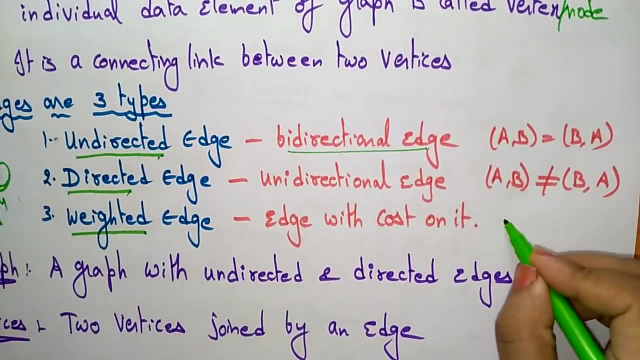 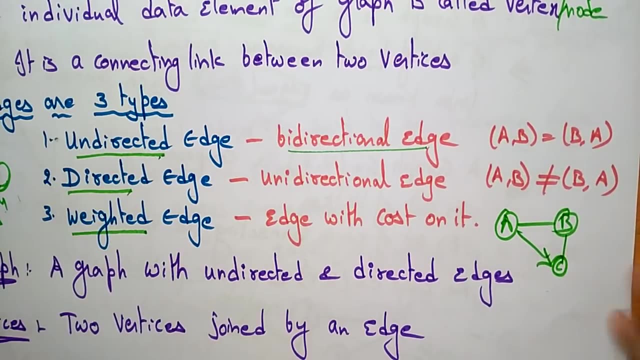 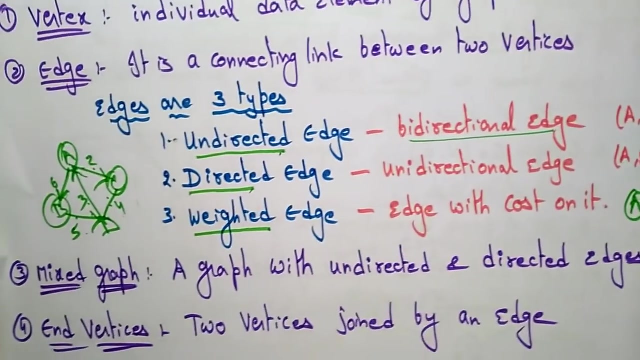 the next terminology, that is a mixed graph, a graph with undirected and directed edges. called mixed graph means both direction will be there and undirection will be there. means, suppose a to b and a to c's direction is there. so this is, this is mixed graph, a graph with undirection and directed edge. next terminology: 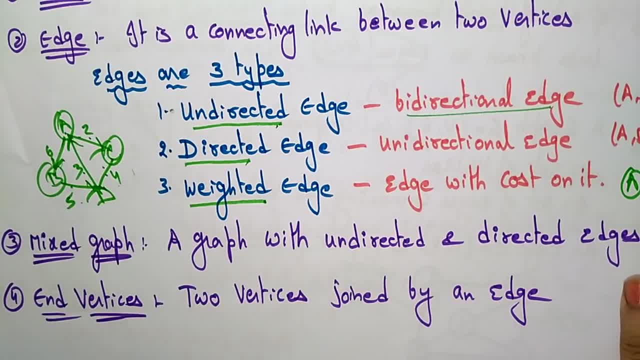 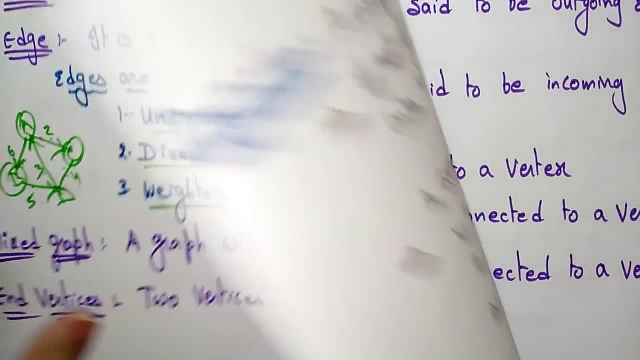 is end vertices. what do you call my end vertices? if two vertices joined by an, by an edge, that you call it as an end vertices? you call it as an end vertices. now, coming to the next terminology, that is, the origin. origin means if an edge is directed. 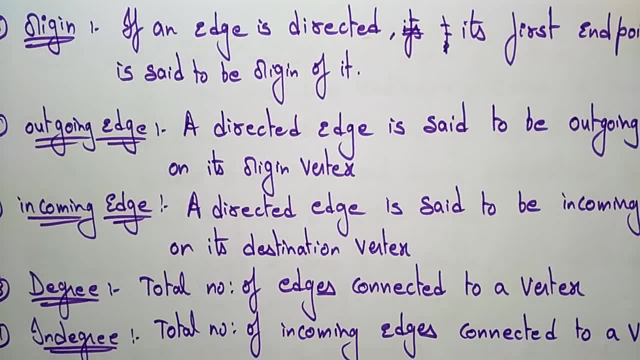 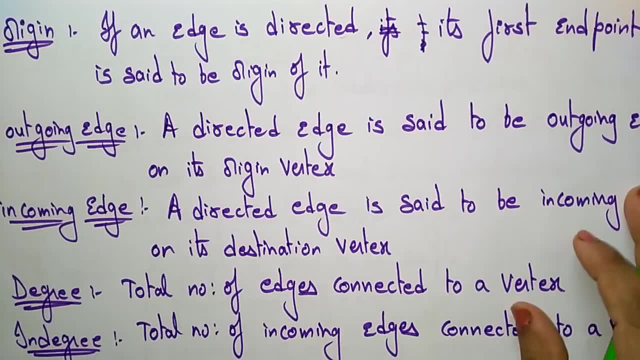 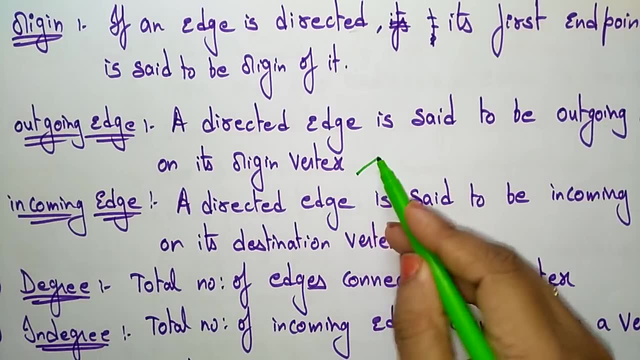 its first end point is said to be origin of it. so whenever your edge is directed then you can find out your origin. so the first end point is said to be the origin of it. outgoing edge: a directed edge is said to be outgoing edge or its origin vertex. so the outgoing edge and 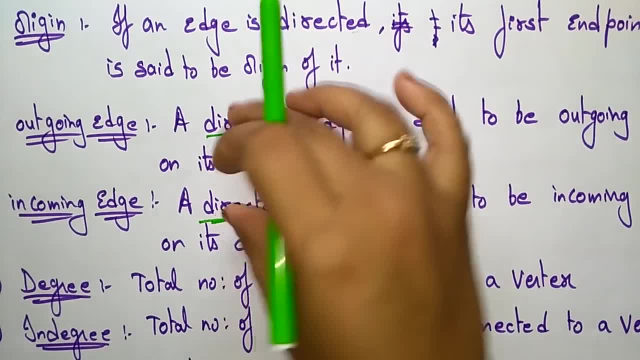 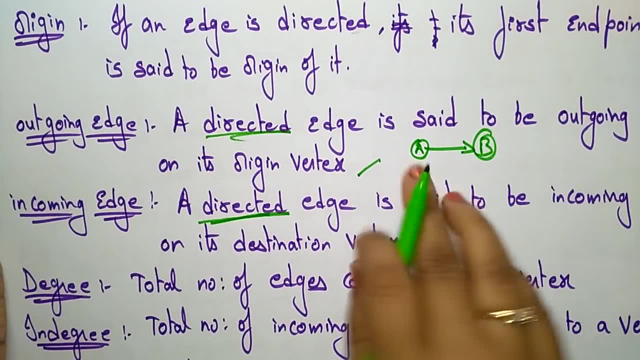 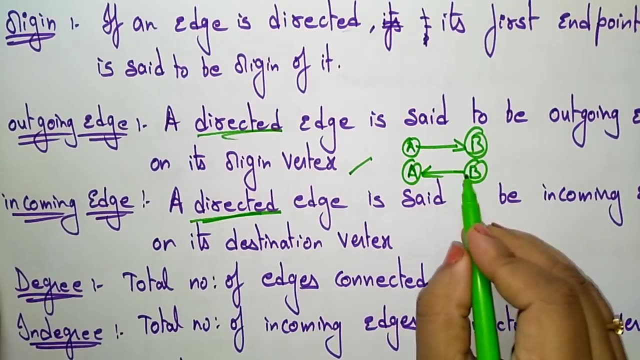 incoming edge should be directed, not unidirected. the both will be directed only so, whenever it is going out from a to b, these you call it as outgoing each. let us take this type of edge, this you call it as incoming edge. so a, the incoming edge and this is outgoing edge. 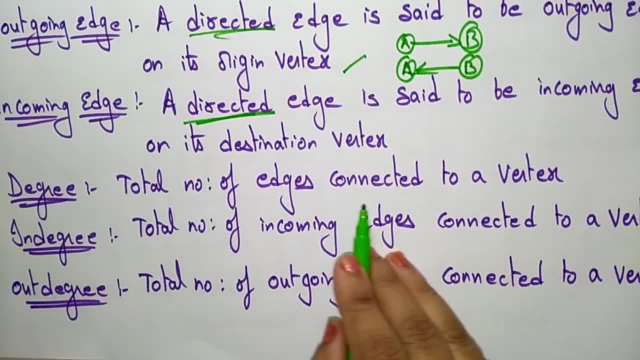 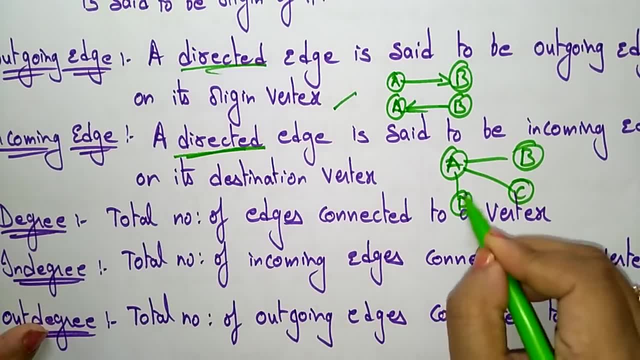 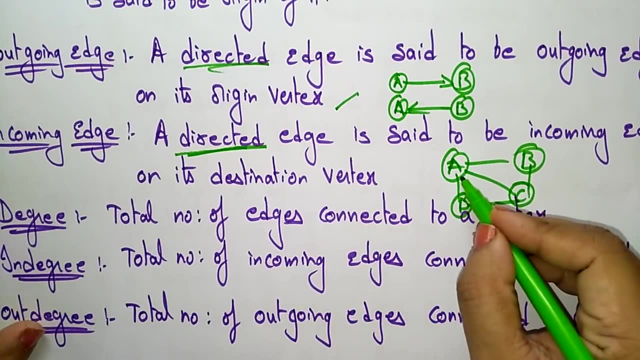 now coming to the degree of edge. degree means total number of edges connected to your vertices. suppose it here: a, b, c, D. This is a graph. So here, what is the degree of? A? The total number of edges connected to a vertex. So to vertex how many edges are connected? 1,, 2,, 3.. So the degree is 3. and for B, how many? 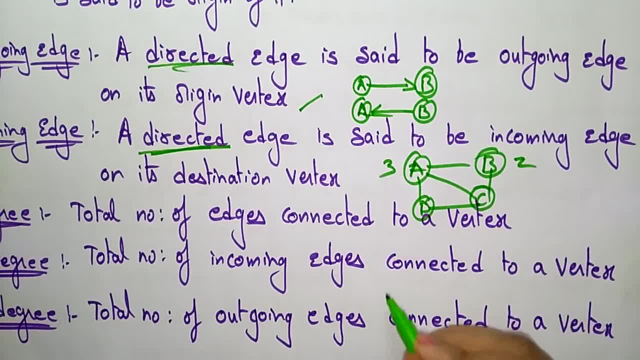 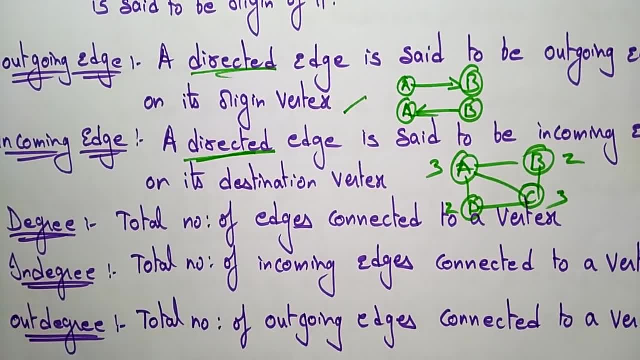 edges will connected to this vertex Only 1, 2.. Degree is 2.. For C, 3 and for D, 2.. So that is where you have to calculate the degree of the vertex. The degree of vertex is nothing but the. 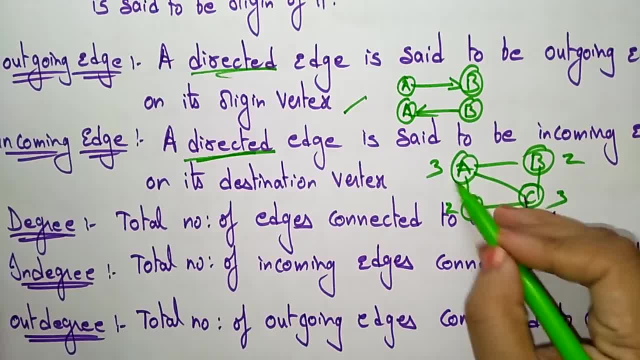 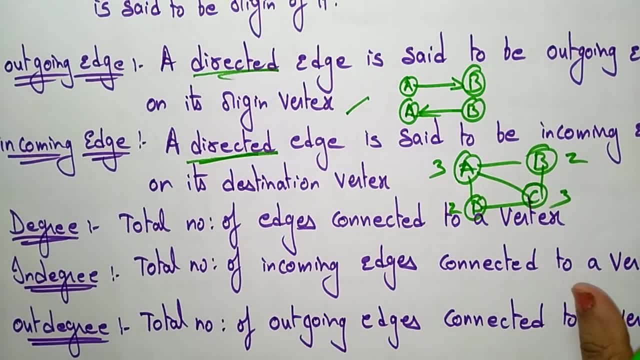 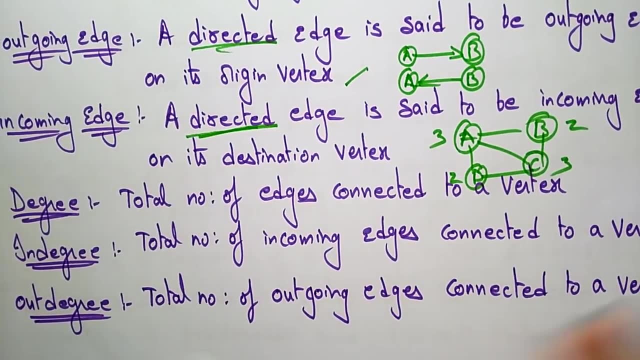 total number of edges connected to a vertex, Whatever the vertex you have taken. So then, edges that are connected to that vertex, you call it as a degree of the edge, That is, the total number. In degree means total number of incoming edges. Out degree means total number of outgoing. 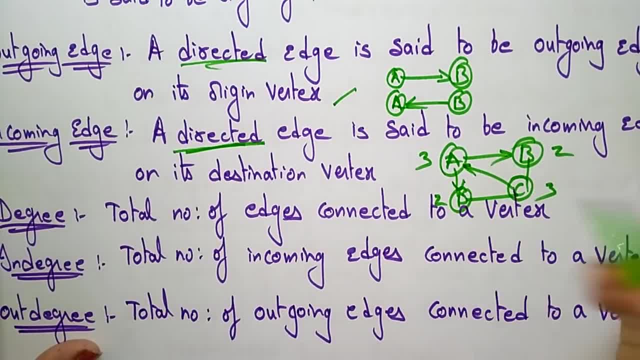 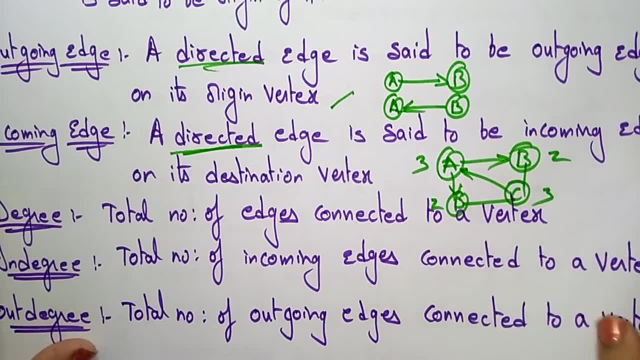 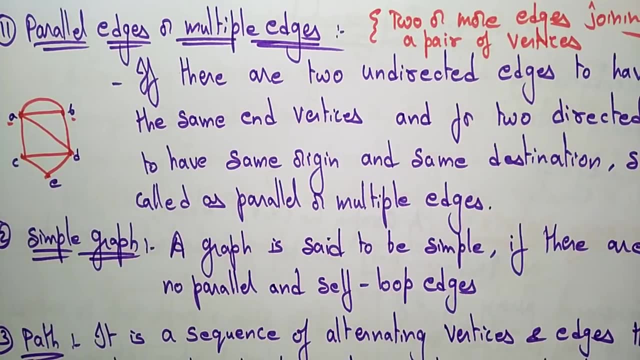 edges, So how many are incoming and how many are outgoing. That is the in degree. So here A is outgoing is 1, 2.. Outgoing is 2, incoming is 1.. And next, coming to the next terminology, that is a parallel edge, or multiple edges, So a parallel. 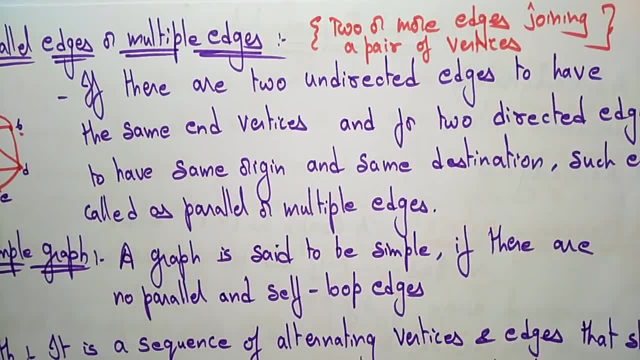 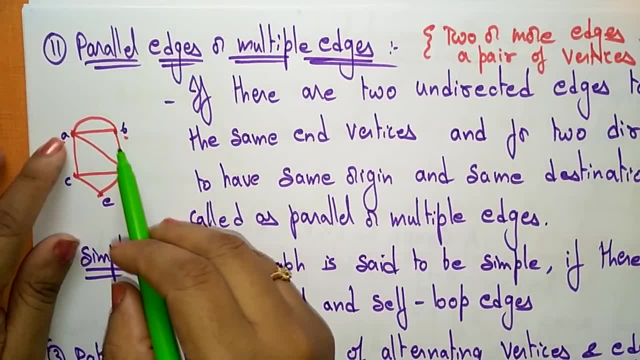 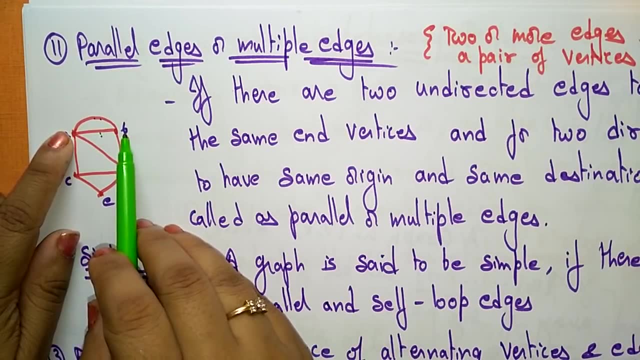 edge is nothing but a 2 or more edges joining a pair of vertices. that you call it as a parallel edge. What it might mean by the 2 or more edges- So here you can see this is in the diagram A- B is having 2 edges, Only for these 2 vertices. you are having the 2 edges, So this you call it.